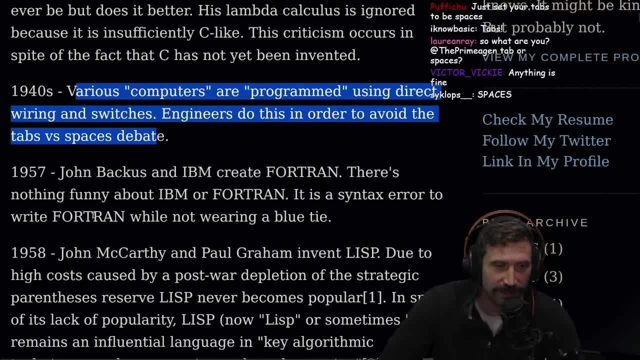 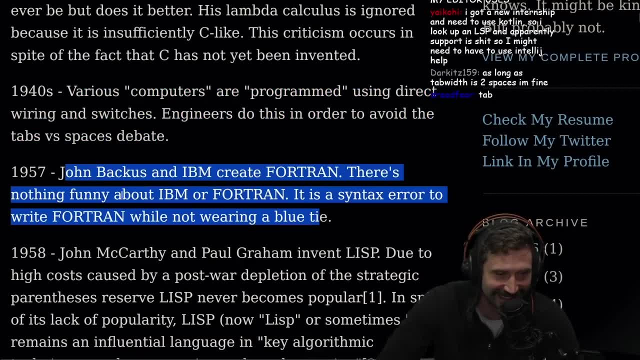 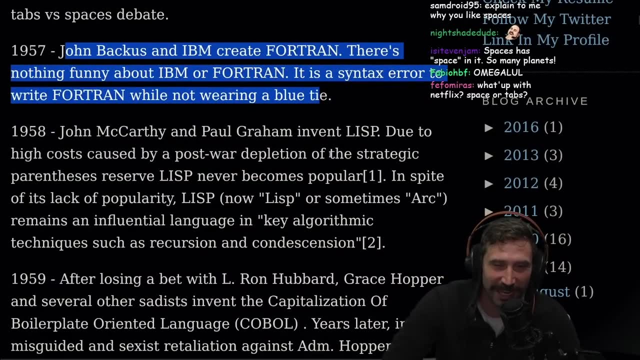 1957.. John Backus and IBM create Fortran. There's nothing funny about IBM or Fortran. It is a syntax error to write Fortran while not wearing a blue tie. That's a pretty good one. John McCarthy and Paul Graham invent Lisp. 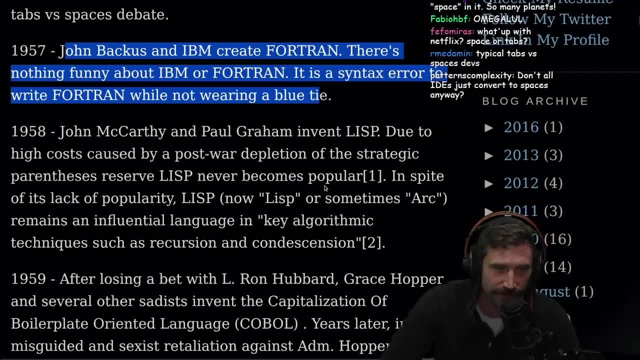 Due to the high cost caused by a post-war depletion of the strategic parentheses reserve, Lisp never becomes popular One. in spite of its lack of popularity, Lisp- now Lisp, or sometimes Arc- remains an influential language in key algorithmic techniques such as recursion and condescension. 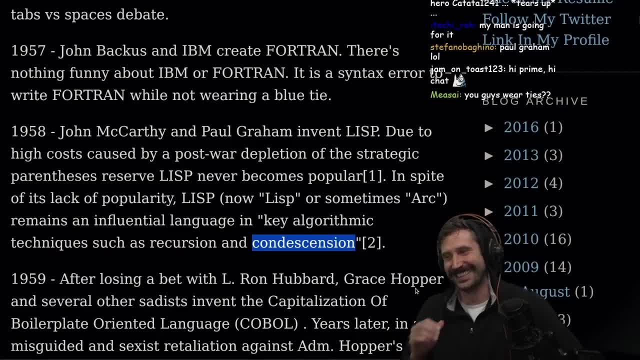 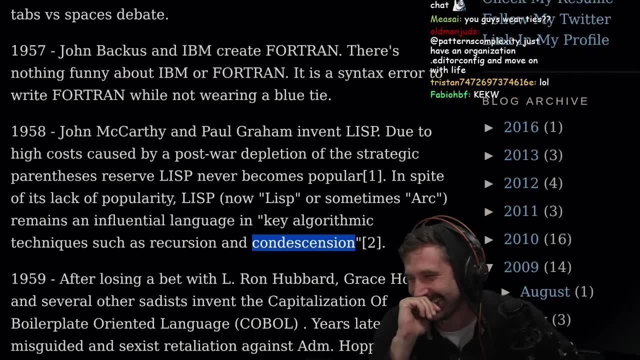 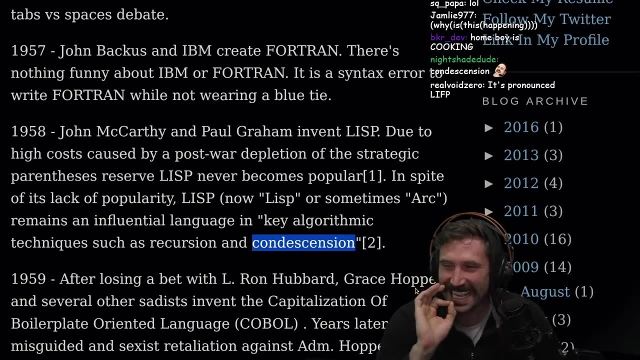 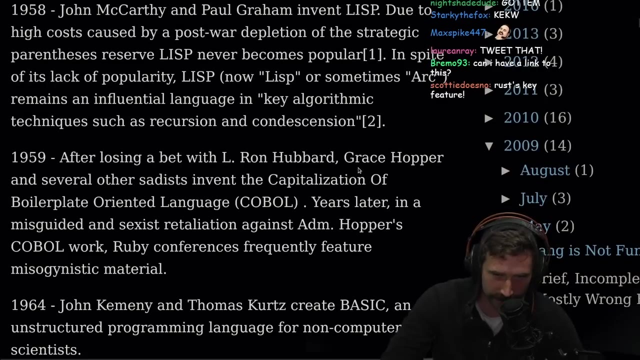 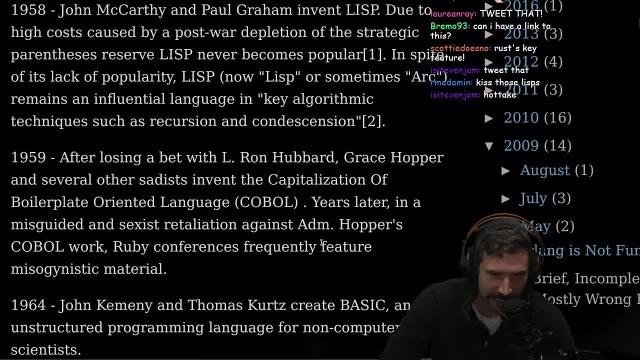 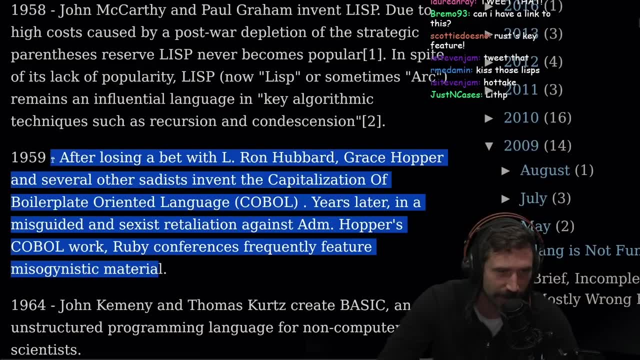 A year later, in a misguided and sexist relation against Admiral Admiral Hopper. COBOL work. Ruby Conference frequently featured misogynistic material. Wait, what did I just read? Is this a dig at DHH? I can't even tell what I just read. 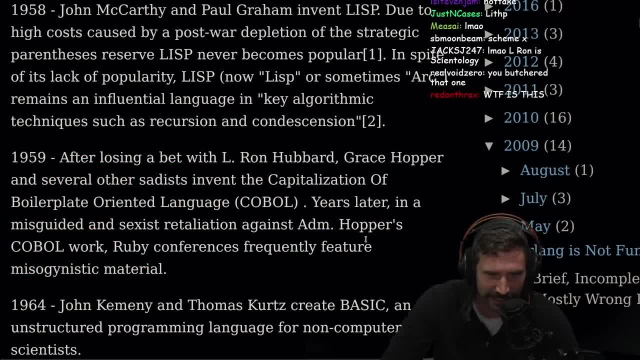 Years later, in a misguided and sexist retaliation against Admiral Hopper's COBOL work, Ruby Conference's frequently featured misogynistic material. What does that even mean? Okay, I must be missing the joke. Is there a joke that I'm missing? 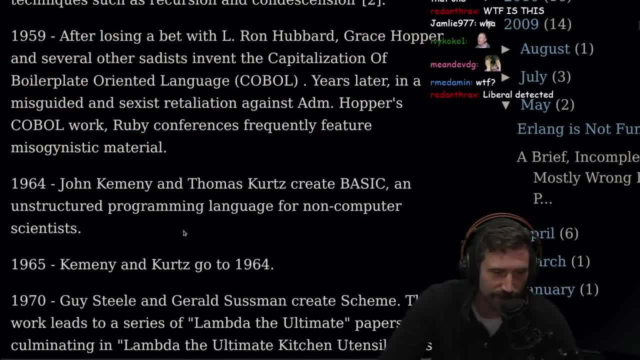 Is this like the Pi Conference, the PiCon 8?, Where some dude Who's like uh, dongle, that doll, you know what I mean? And then boom, the internet blows up and there's never been a conference the same sense. 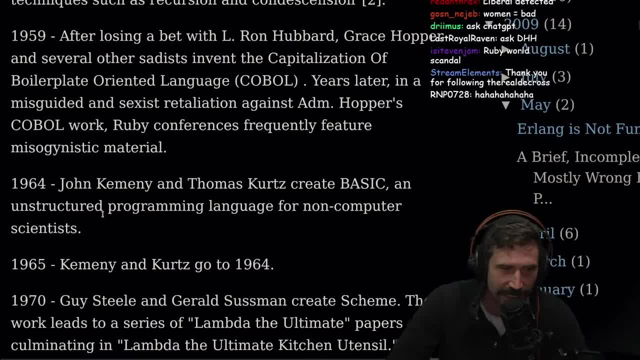 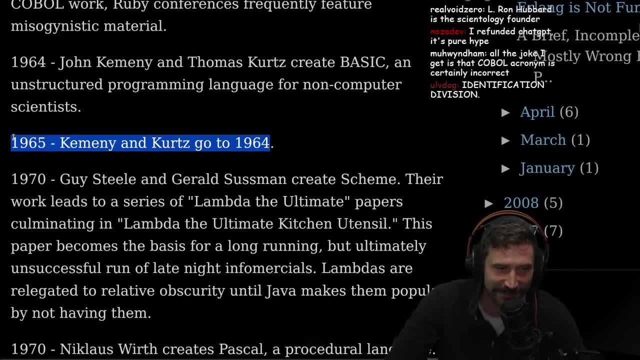 John Kemeny and Thomas Kurtz create BASIC, an unstructured programming language for non-computer scientists, 1965.. Kemi and Kurtz go to 1964.. It's pretty good, Guy Steele and uh Gerold. 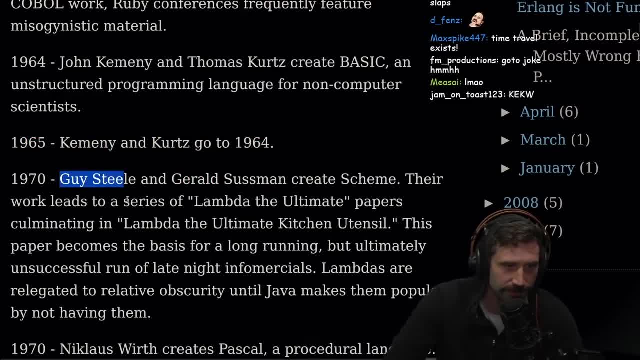 Gerold Ooh, Gerold of Riviera, Uh, Gerold Steele and Oh uh Guy Steele. Guy Steele and Gerold Sussman create Scheme. Their work leads to a series of Lambda- the ultimate papers- culminating in Lambda- the ultimate kitchen utensil. 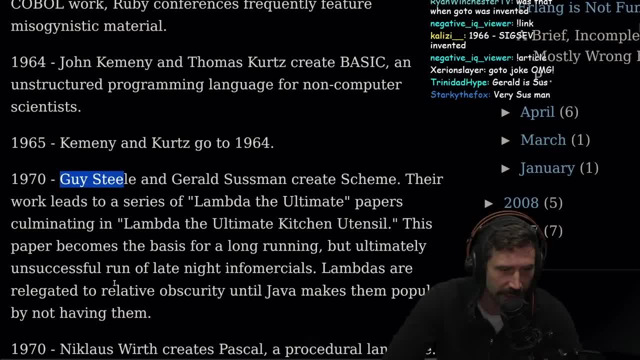 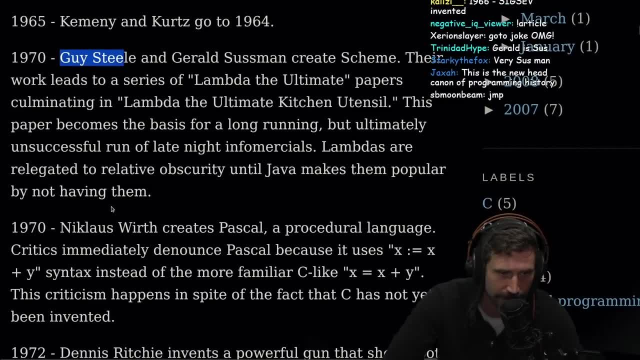 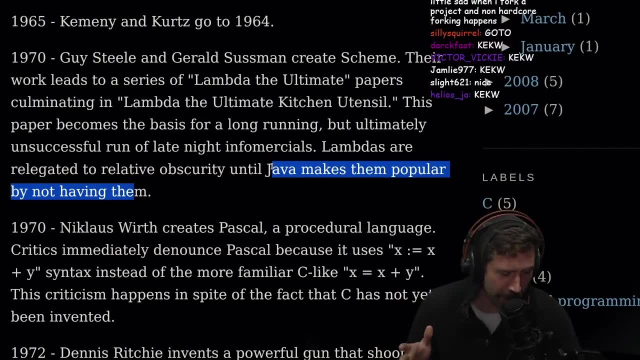 This paper becomes the basis for long-running but ultimately unsuccessful run of late-night infomercials. Lambdas are relegated to relative obscurity until Java makes them popular. by not having them, I mean you. technically you get them, You just create an interface with a method that you call back. 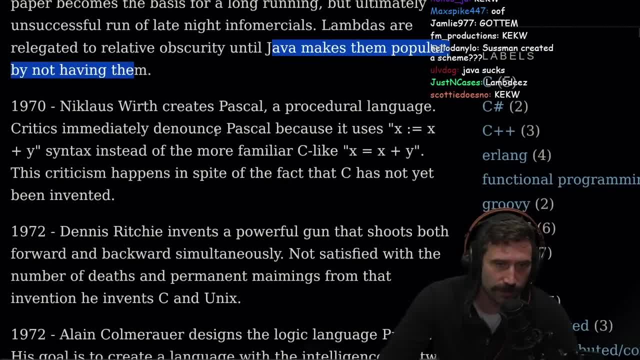 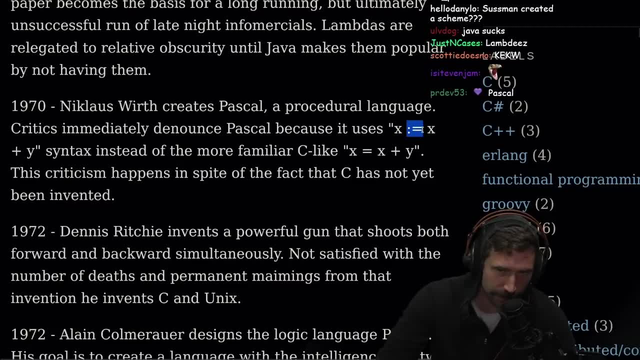 Uh. in 1970.. Nicolas O'Worth creates Pascal, a procedural language. Critics immediately denounce Pascal because it uses X- uh, bad guy from Turok 2, X plus Y syntax instead of the more familiar C-like interface. uh, C-like X equals X plus Y. 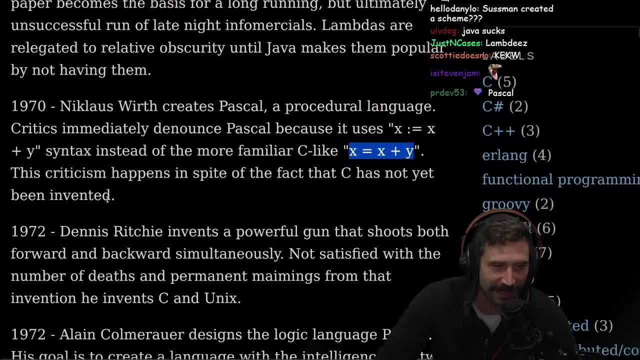 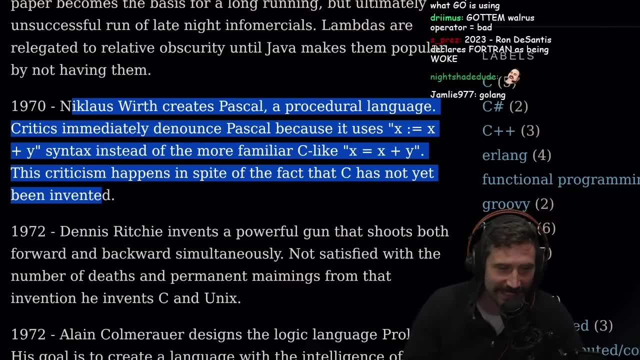 This criticism happens in spite of the fact that C has not been invented yet. You know why is C just the the? why does C feel like the right way? Why? why is it? Why? Why does C win? Dennis, uh, Ricky, uh, Richie uh, invents a powerful gun. 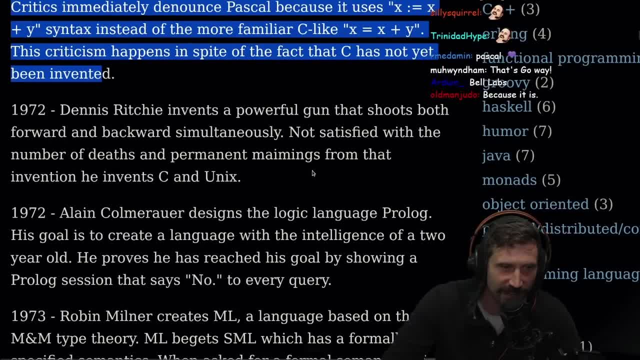 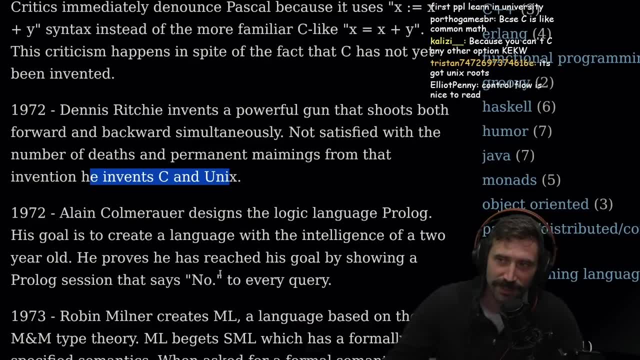 That shoots both forward and backwards simultaneously. Not satisfied with the number of deaths and permanent maimings from that invention, He invents C and Unix. I mean, it's pretty good See. the problem is it only kills two people at a time if both shots hit. 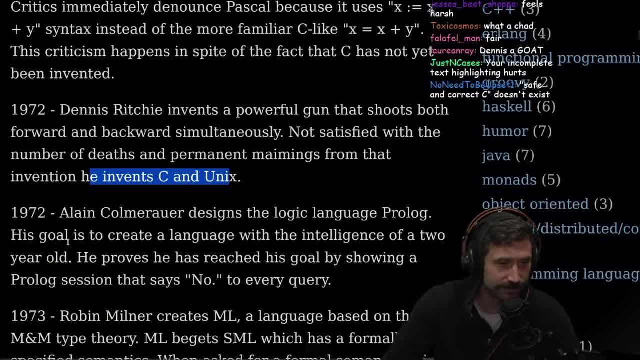 That's only if both shots hit. You know what I mean. That means if you shoot it like Arnold, you're gonna die. Uh, let's see. Uh, Alain, uh, Colm, uh, do I even know how to say this name? 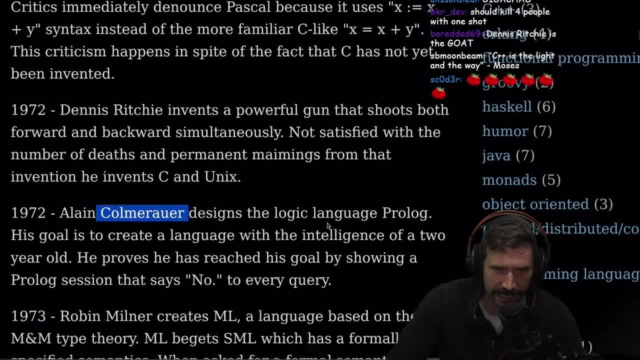 Alain Colmerier designs the logic pro uh language prologue. His goal is to create a language with the intelligence of a two-year-old. He proves that he has reached his goal by showing a prologue session that says no to every query. 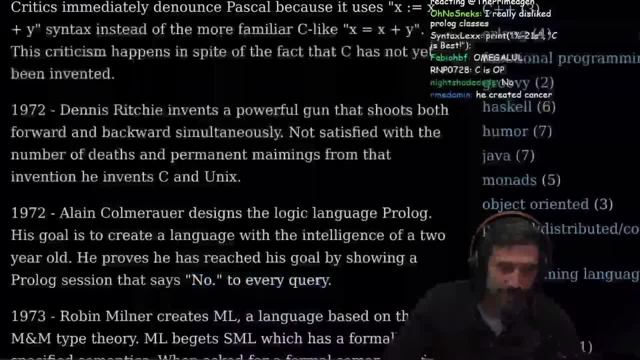 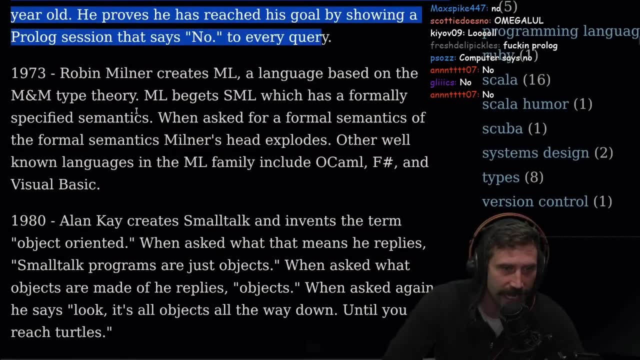 Let's go. That is so correct. That joke is way more funny now that I've had four kids. Uh, Robin Milner creates ML, a language based on the M&M type theory. ML begets SML, which has a formally specified semantics. 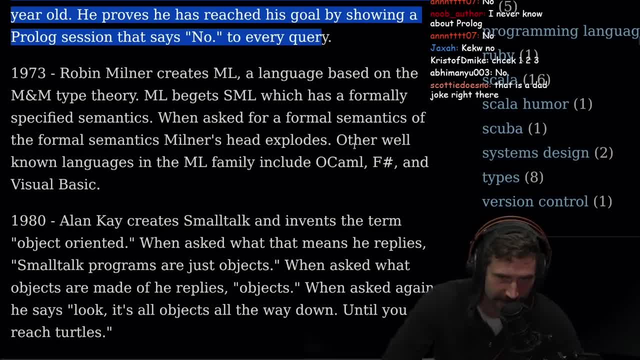 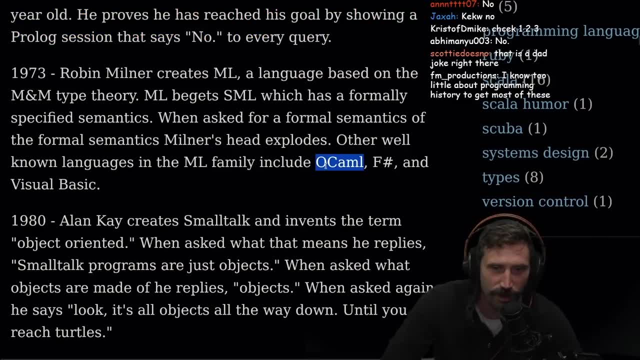 When asked for a formal semantics of the formal semantics, Milner's heads explodes. Other Other well-known languages in the ML family, including OCaml, F-Sharp and Visual Basic. Let's go OCaml, We got an OCaml mention. 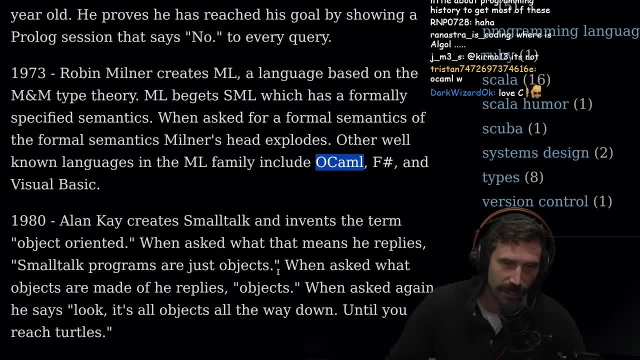 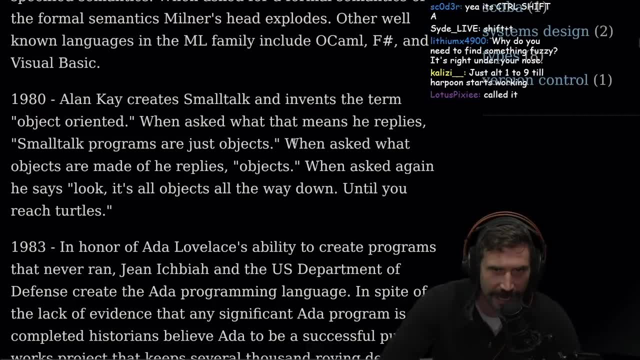 Let's go. If I, if I had the time to program any language I'd want right now, I OCaml would be the language. In 1980, Alan Kay creates Smalltalk and invents the term object-oriented. When asked what it means, he replies: Smalltalk programs are just objects. 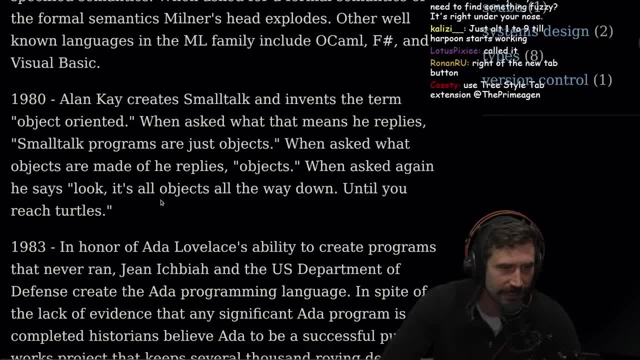 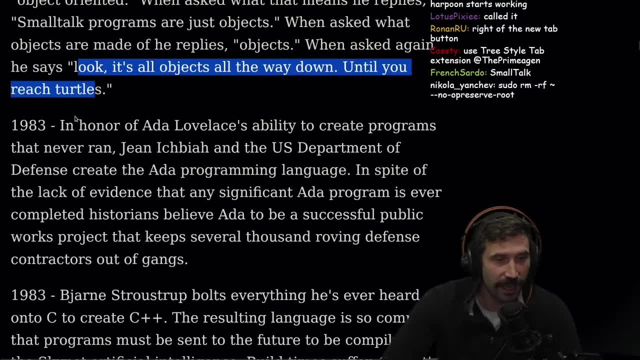 When asked what objects are made of, he replies objects. When asked again, he look. he says look, it's all objects all the way down until you reach turtles. It's a fair statement- I like turtles- In honor of Ada Loveless's ability to create programs that never ran. 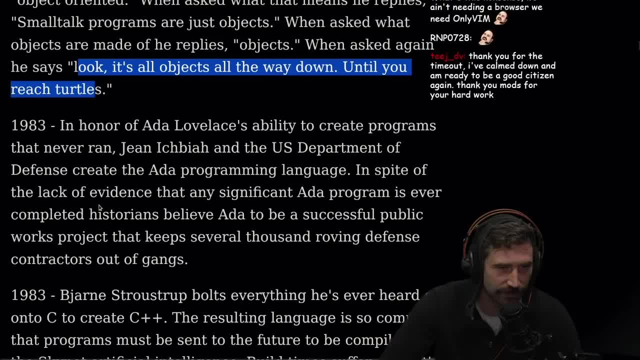 John Ichbach and the US Department of Defense creates Ada programming language. In spite of the lack of evidence that any significant Ada program is ever completed, historians believe Ada to be a successful public works project that keeps several thousand roving defense contractors out of gangs. 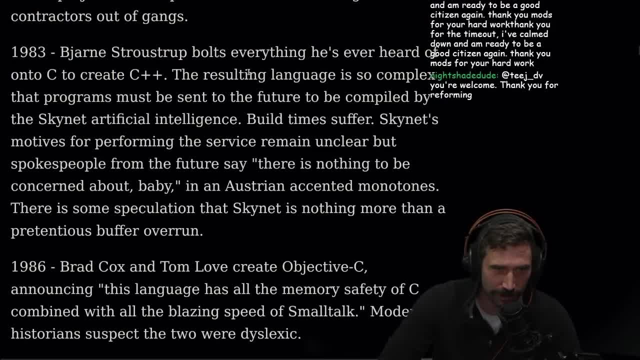 Oh no, In 1983, Bjarn Strasser, Strasser, Strasser Bolts everything he's ever heard of onto C and creates C++. The resulting language is so complex that programs must be sent to the future to be compiled by Skynet Artificial Intelligence. 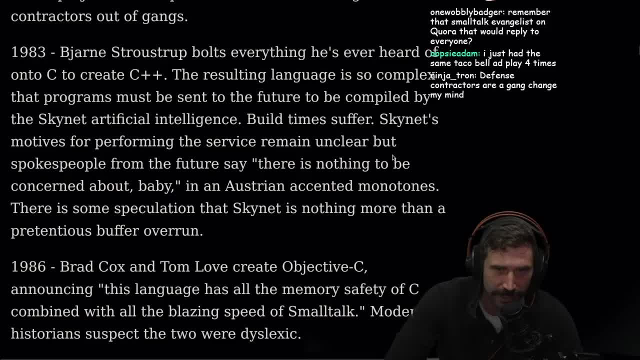 Build times suffer. Skynet's motives for performing the service remain unclear, but spokespeople from the future says there is nothing to be concerned about baby. In an Australian accent monotones: In an Austrian accent monotones: There's nothing to be concerned about baby. 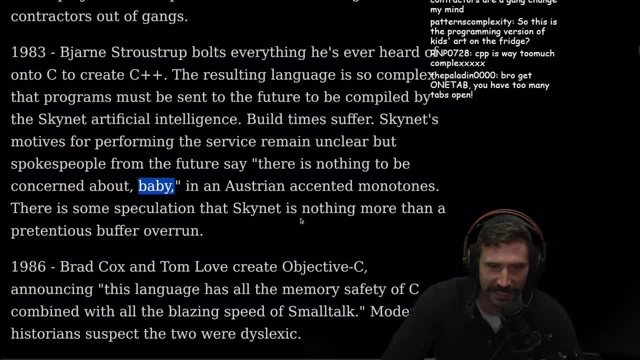 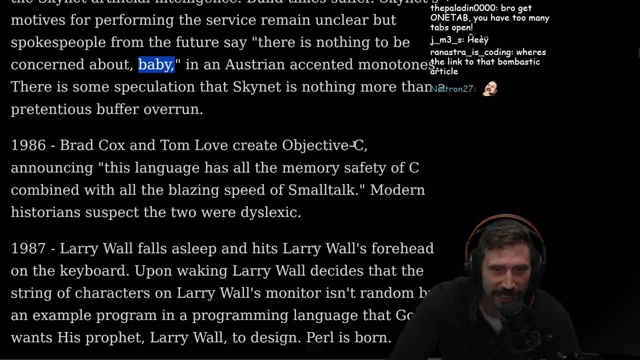 There is some speculation that Skynet is nothing more than a pretentious buffer. overrun 1986,, Brad Cox and Tom Love create Objective-C. announcing this language has all the memory safety of C combined with all the blazing speed of small talk. Modern historians suspect the two were dyslexic. 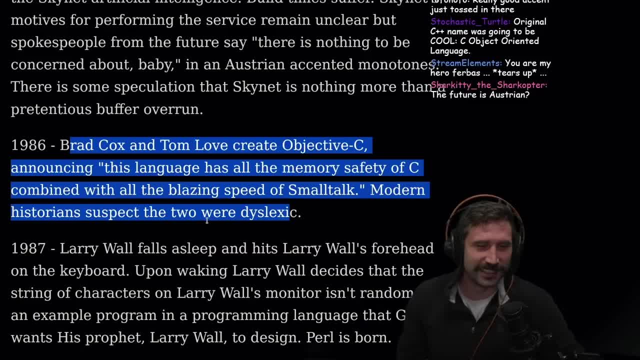 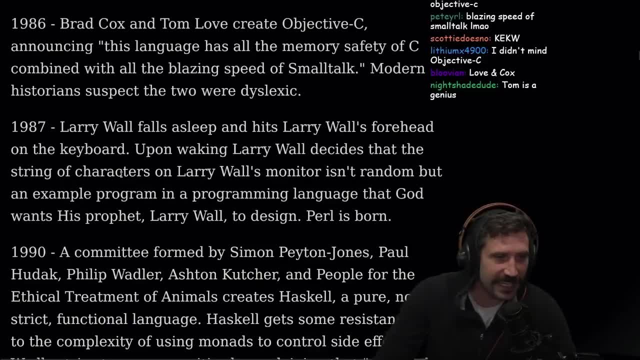 As someone who's done a decent amount of Objective-C. this is a. This is a great statement. This is a great statement. okay, This is beautiful. In 1987, Larry Wall falls asleep and hits Larry Wall's forehead on the keyboard. 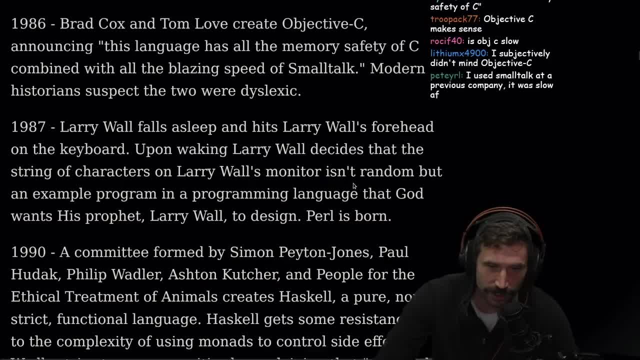 Upon waking, Larry Wall decides that the string of characters on Larry Wall's monitor isn't random, but an example program in a programming language that God wants his prophet Larry Wall to design: Pearl is born. This is an actual, factual statement. okay, 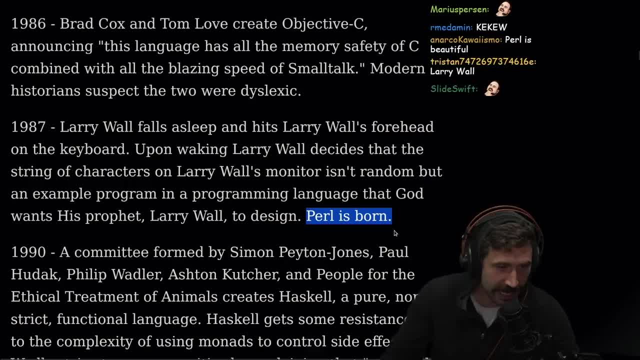 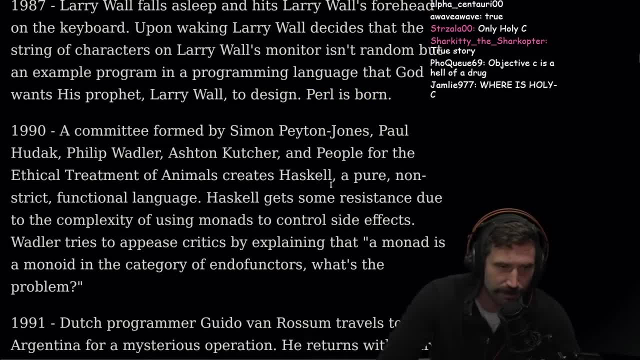 This is not a mostly incorrect. This is actually a very correct statement. In 1990,, a committee formed by Simon Payton Jones, Paul Haddock, Philip Wadler, Ashton Kutcher and the people for the ethical treatment of animals create Haskell. 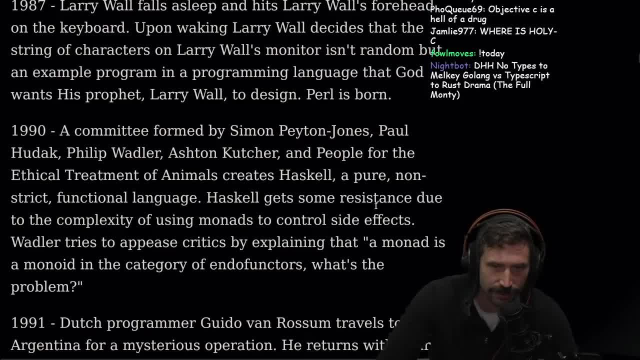 a pure, non-strict, functional language. Haskell gets some resistance due to the complexity of using monads to control side effects. Walter tries to appease critics by explaining that a monad is a monoid in the category of endofunctors. 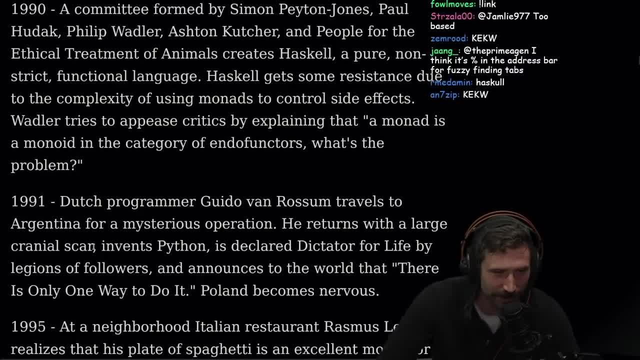 What's the problem? Dutch programmer Guido van Rossum travels to Argentina for a mysterious operation. He returns with a large cranial scar and Fence Python is declared dictator for life by legions of followers and announces to the world there is only one way to do it. 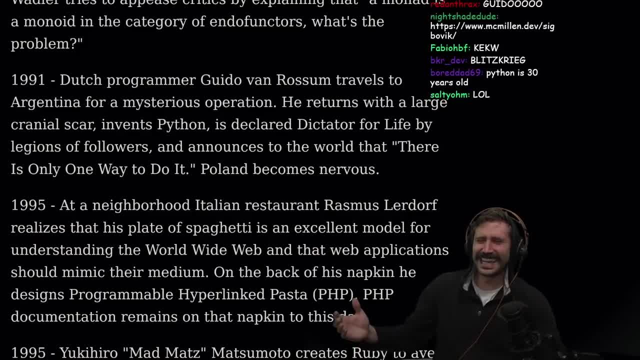 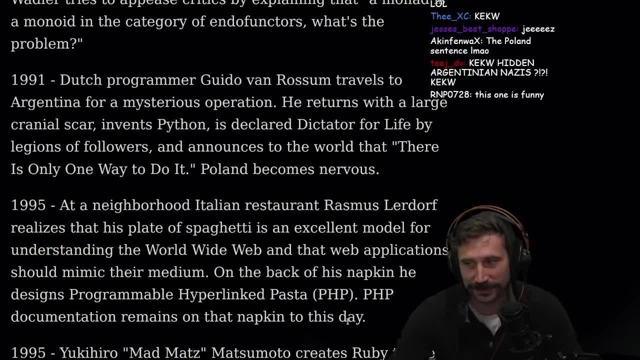 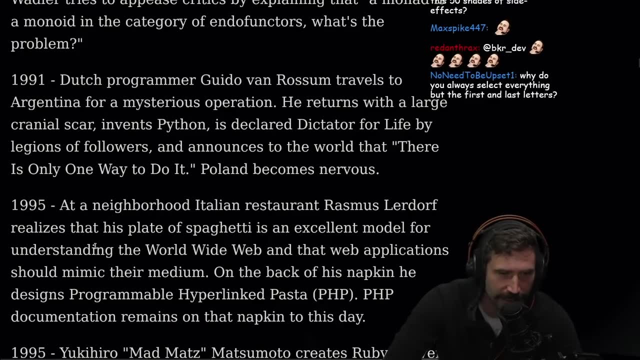 Poland becomes nervous. What did I just read? What phrase just came out of my face hole? That one was pretty good, though I'll give it It's pretty good. In 1995, at a neighborhood Italian restaurant, Rasmus Lurdorf realizes that his plate of spaghetti is an excellent model for understanding the World Wide Web. 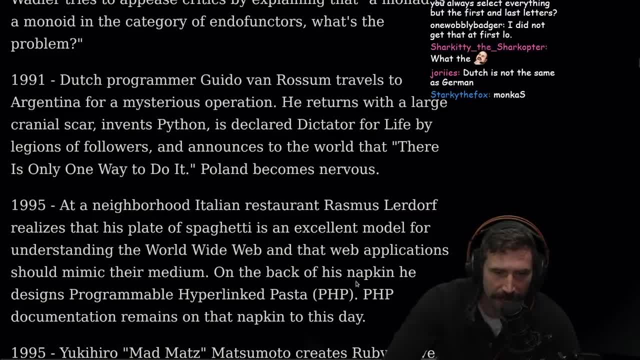 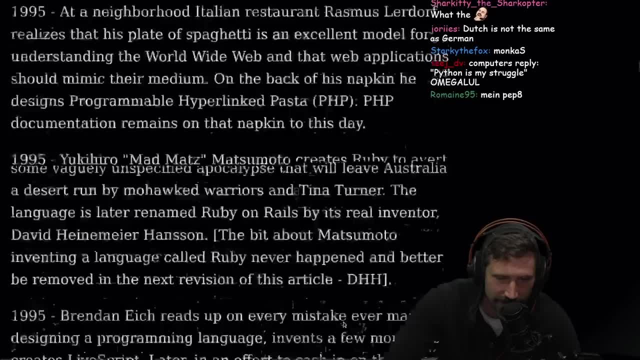 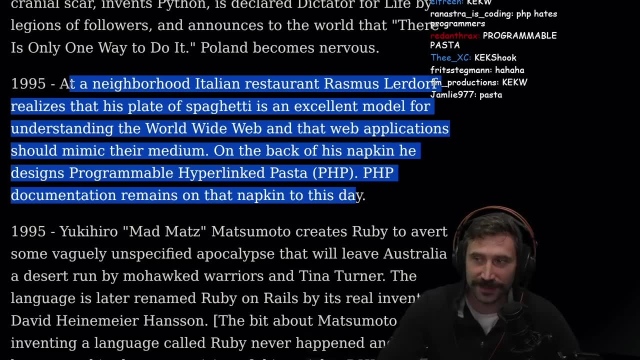 and that web applications should mimic their medium. On the back of his napkin he designed programming programmable hyperlink pasta, PHP. PHP documentation remains on that napkin to this day. Taylor Otwell shook. right now, Taylor is shook. What they forgot to say is that napkin is also in a Lamborghini. 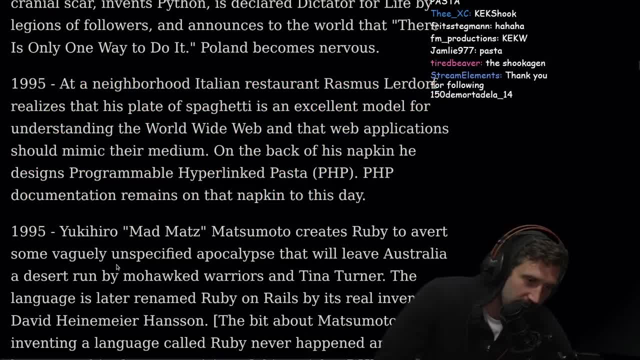 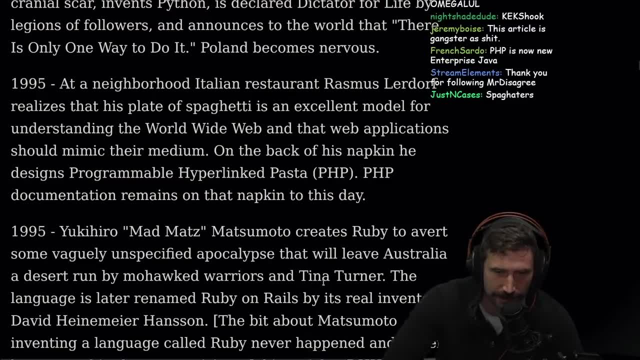 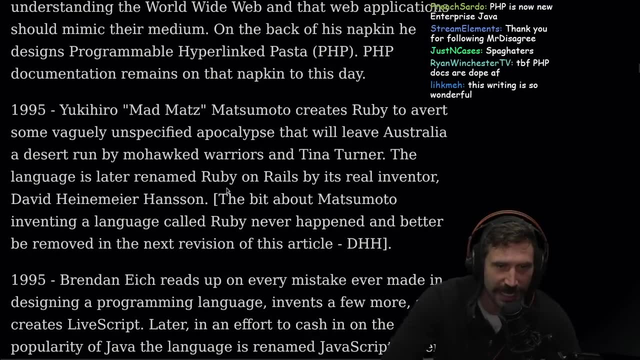 So it's like. you know how bad is it? Yukihiro Matsumoto creates Ruby to advert some vaguely unspecified apocalypse that will leave Australia a desert run by mohawked warriors and Tina Turner. The language is later renamed Ruby on Rails by its real inventor, David DHH. 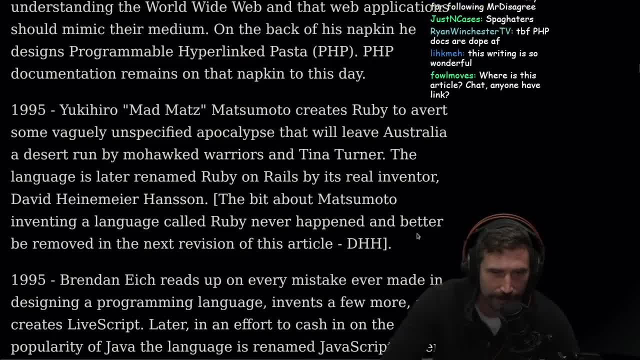 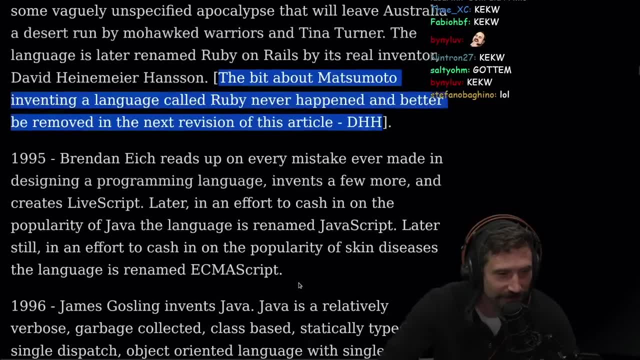 The bit about Matsumoto inventing a language called Ruby never happened and better be removed in the next revision of this article. DHH, the man loves not having types. In 1995, Brendan Eich reads up on every mistake ever made designing a programming language. 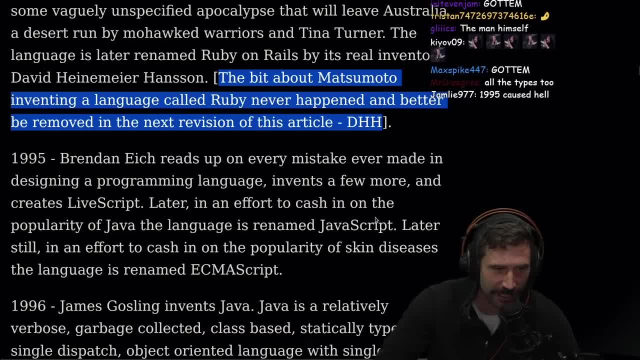 invents a few more and creates LiveScript. Later, in an effort to cash in on the popularity of Java, the language is renamed to JavaScript. Later, still in an effort to cash in on the popularity of a skin disease, the language is renamed ECMAScript. 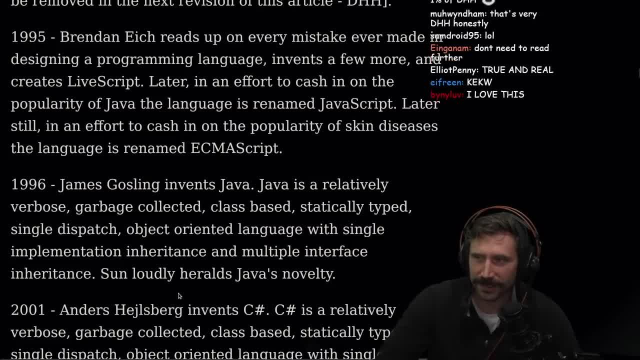 That's actually a pretty accurate statement right there. That's just reality. 1996, James Gosling invents Java. Java is relatively verbose: garbage collected class-based. Wait, hold on. How did Brendan Eich invent? Oh, later on it's renamed. 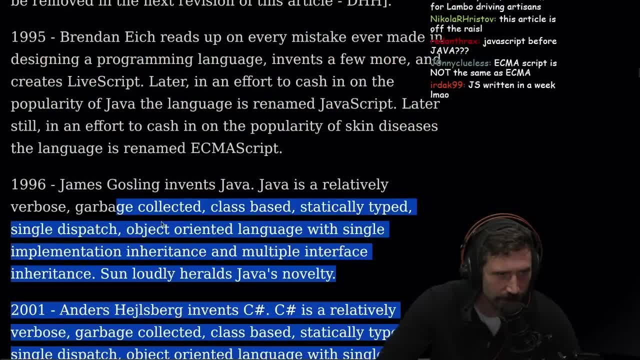 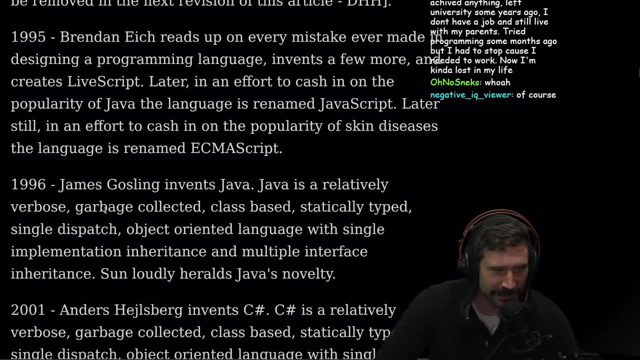 Okay wait, did JavaScript appear before Java? I know this is mostly incorrect, I know this is an incorrect history, But JavaScript came out before Java. This has to be a troll, Because Null, yeah, it has to be a troll. 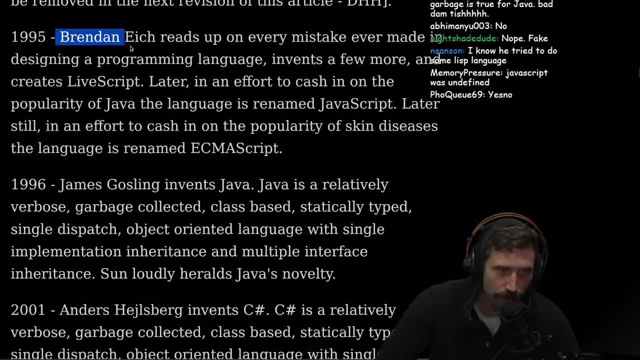 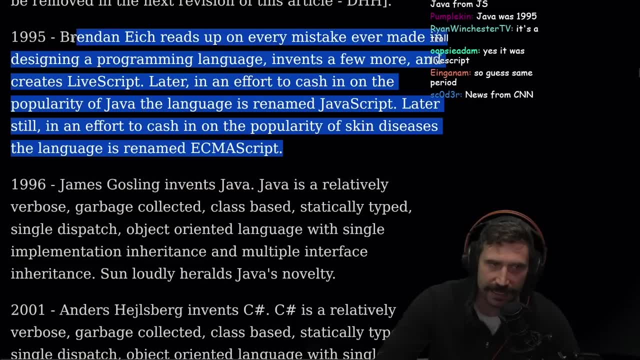 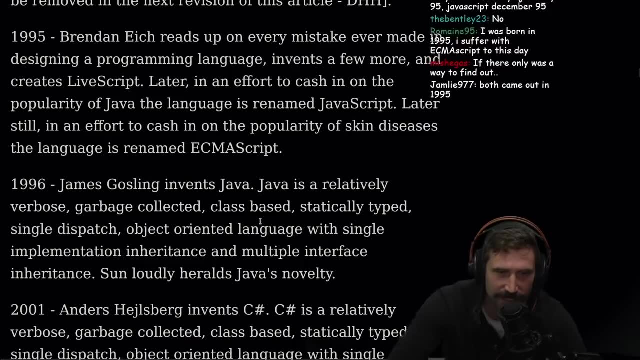 Because Null from Brendan Eich's own mouth is that he had to do Null because of Java. So it has to, it cannot be. It cannot be. news from CNN: James Gosling invents Java. Java is relatively verbose: garbage collected, class-based, statically typed, single dispatch. 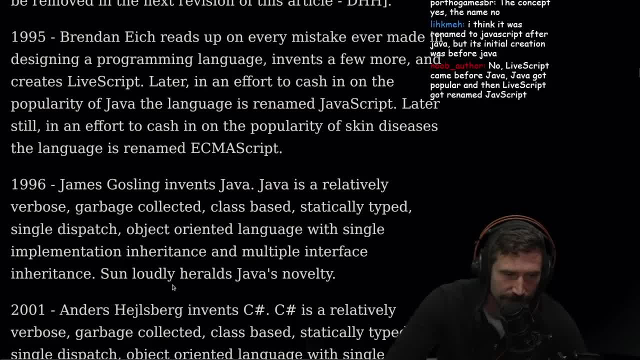 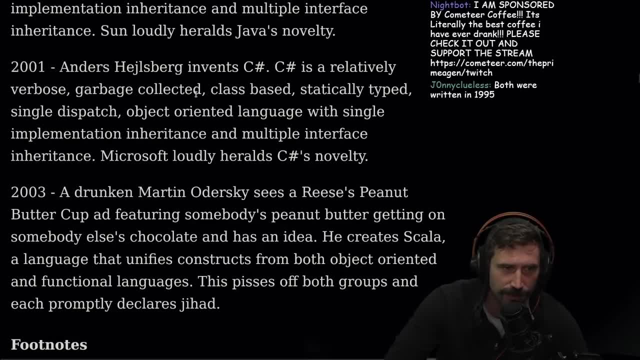 object-oriented language with single implementation inheritance and multiple interface inheritance. Sun loudly heralds Java's novelty. Anders Heilsberg invents Csharp. Csharp is a relatively verbose garbage. collected class-based, statically typed, single dispatch. object-oriented language with single implementation inheritance. 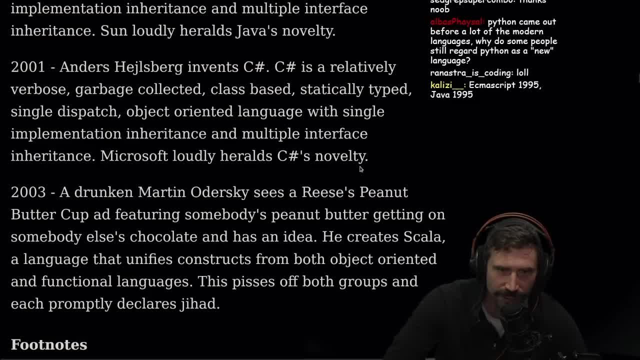 and multiple interface inheritance. Microsoft loudly heralds Csharp's novelty 2003,. a drunken Martin Odeski sees Reese's Peanut Butter Cup ad featuring somebody- peanut butter- getting on somebody else's chocolate, and has an idea: He creates Scala, a language that unifies constructs from both object-oriented and functional. 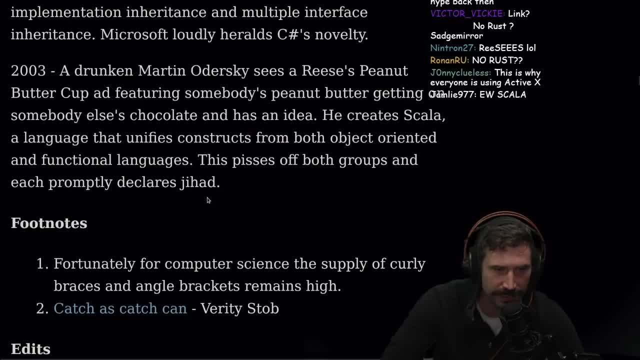 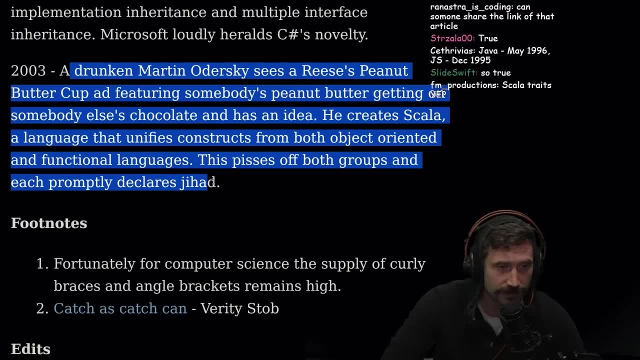 languages. This pisses off both groups and each promptly declares jihad. That's actually pretty accurate. I feel like nobody likes Scala, Except for people that like Scala, But nobody likes people that like Scala. I don't want to teach my kid to code. 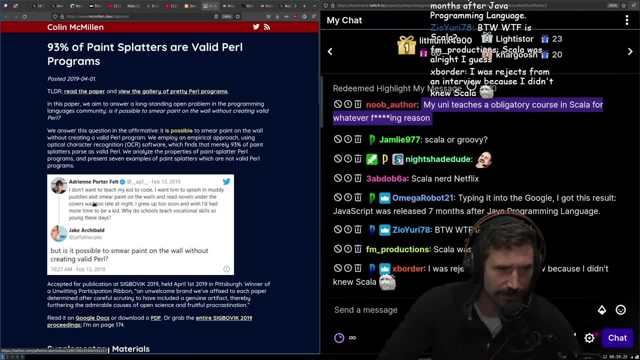 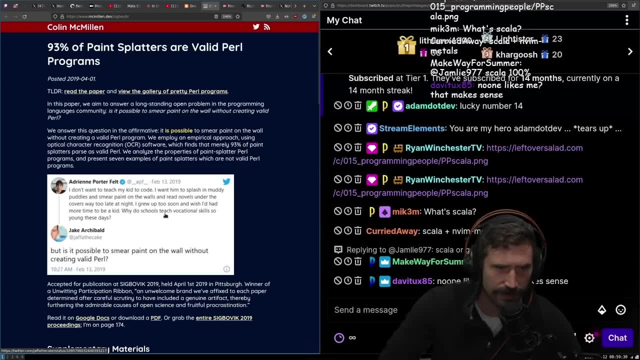 I want him to splash in muddy puddles and smear paint on the walls and read novels under the covers way too late at night. I grew up too soon. I wish I had more time to be a kid. Why do schools teach vocational skills so young these days? 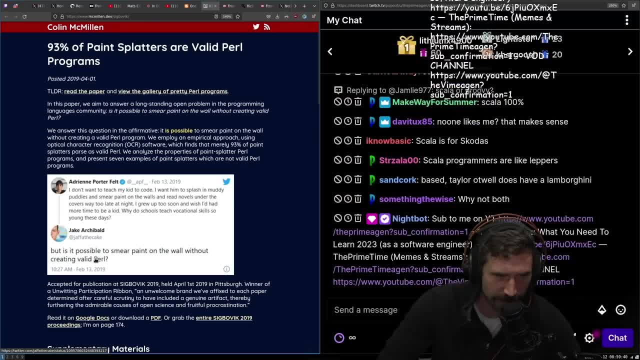 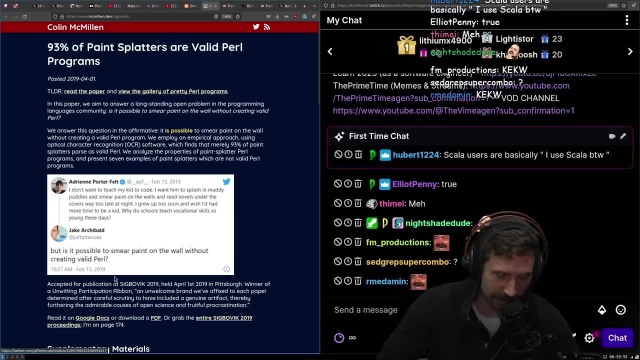 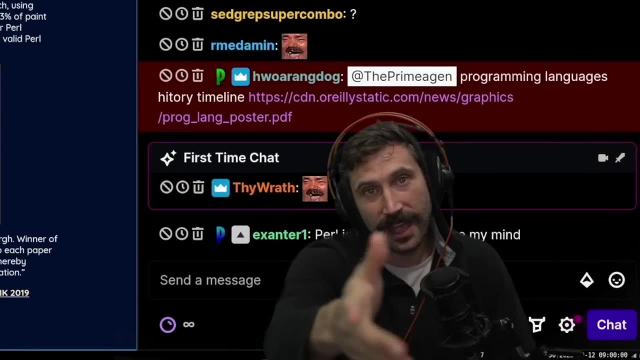 But is it possible to smear paint on the walls without creating valid Perl Based Jake Archibald? First off, your name is like a comic, as it is, And your response is poetic. The name, It's probably a valid programming language. 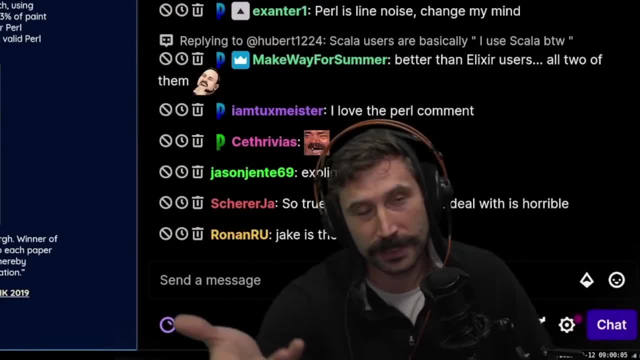 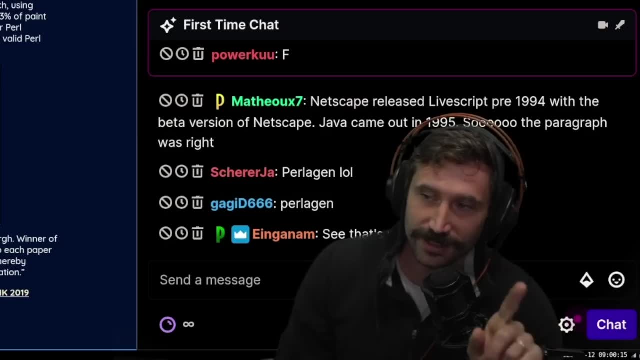 I mean, it's probably a valid programming language. It's probably a valid Perl program. Where did I get programming language from? What's wrong with my brain? Hey, the Perligen: She wears a Perligen necklace. I think I need to end the video now.